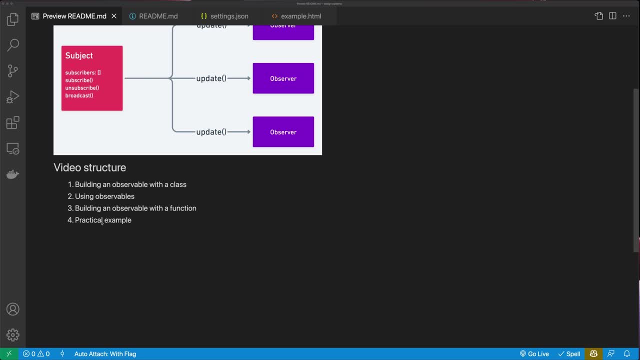 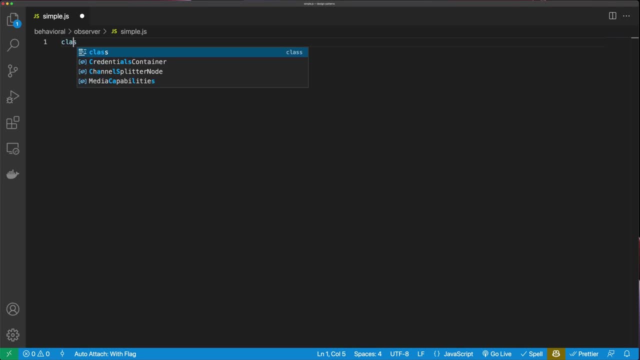 And then, finally, we're going to see a practical example of where you might use observables. So the first thing we need to do to create our observable is to create a class. So I'm going to say class, observable, And inside of the constructor we're going to have 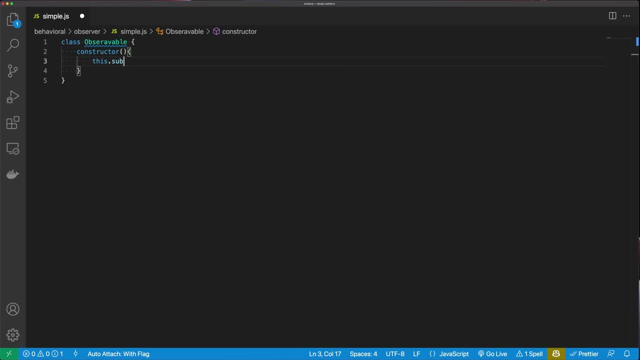 a list of subscribers. So I'm going to say this: dot subscribers. This is an empty array. This method is going to update the list of subscribers. in the first, The first method we're going to have is a subscribe method that will update the list of subscribers. I'm going to say subscribe. 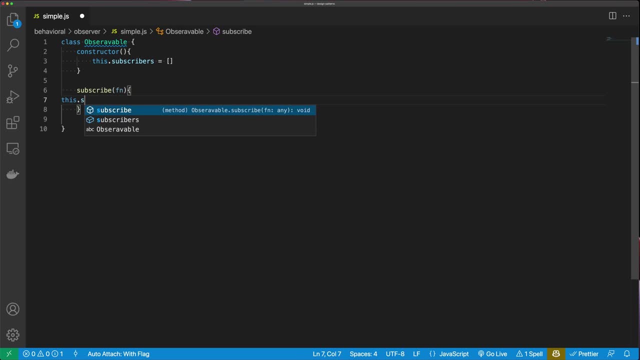 And our subscribe method is going to take a function. Then we're going to say this: dot subscribers, dot push. And we're just going to push our function onto the subscriber list. The next method we're going to have is an unsubscribe method. so I'm going to say unsubscribe. 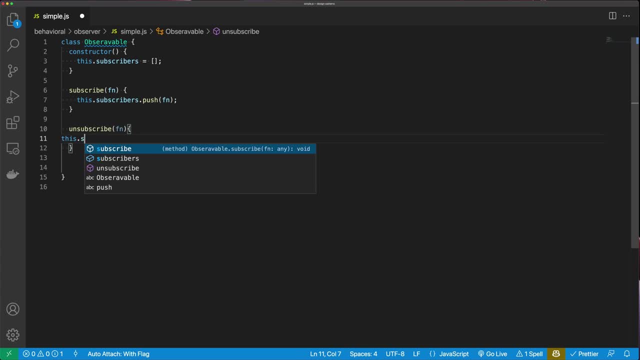 Unsubscribe is also going to take a function and then I'm going to say thissubscribers is equal to thissubscribersfilter item and I'm going to say item is not equal to the function. So we're just going to return a new list of subscribers with the function. 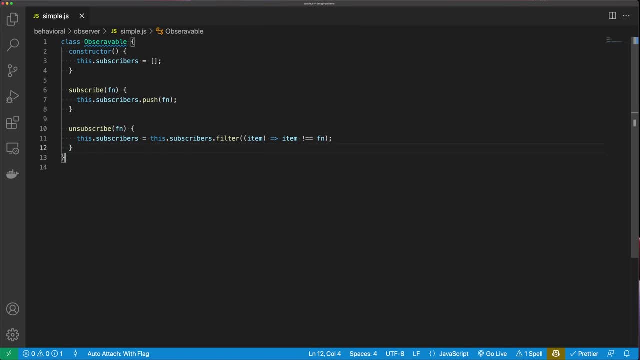 that is going to unsubscribe emitted from that list And then finally, this is where the magic happens. We're going to have a broadcast method, and you might see the broadcast method called other things, such as fire, and what they actually mean is just broadcast out to. 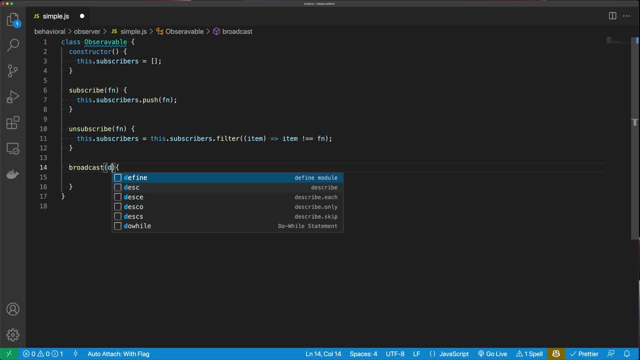 all the subscribers. Broadcast is going to take some data and then we're just going to loop through all of our subscribers and we're going to execute their function with our data. We're going to say for let i equals 0, i is less. 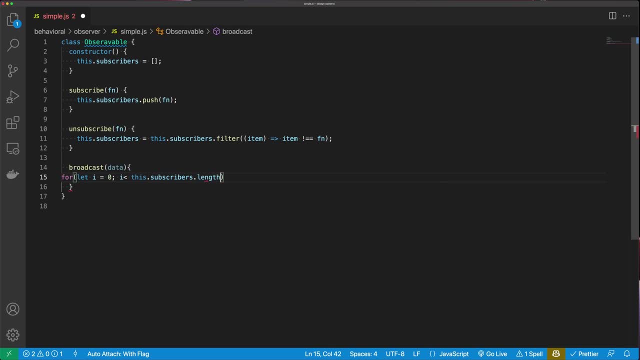 than thissubscriberslength i++, then we're going to say thissubscribers i and then we're going to execute that function with our data. Okay, so you can see how simple an observable is. Let's go ahead and use this observable. So I'm going to say: const observer equals new. 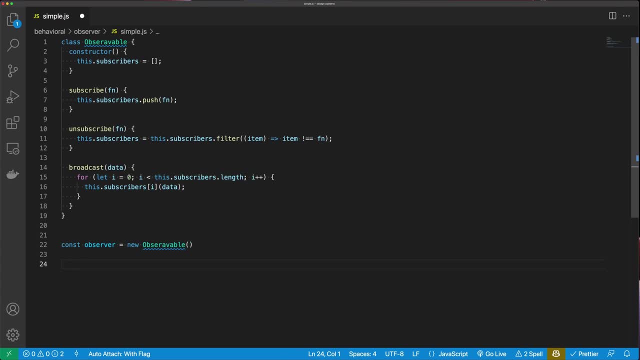 observable. I'm going to say const fn is equal to- and this is just our callback function and it's going to take some data. So when our callback function is executed it's just going to say consolelog: callback was executed. Next we want to say observersubscribe and we want to subscribe with our callback function. 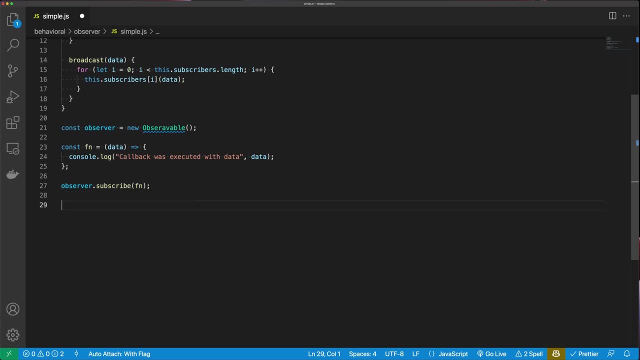 Okay, so let's broadcast some data out to our observable. So I'm going to call observerbroadcast and I'm going to broadcast a message of hello from the observable. What we expect to happen is our observer be created. then we call subscribe with our callback function and then we broadcast. 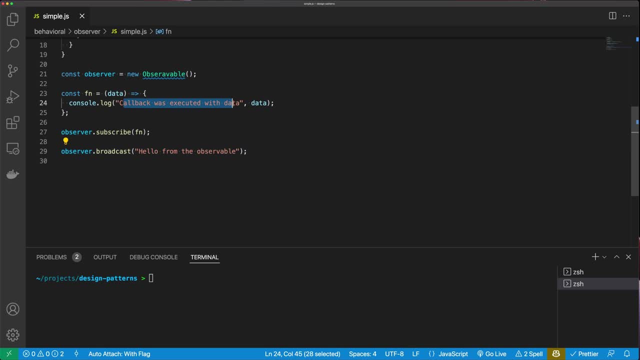 a message, and so we should see a message in the console that says: callback was executed with data hello from observable. and that's exactly what we see: callback was executed from data hello from observable. so let's recreate this observable, but let's do it with a function. 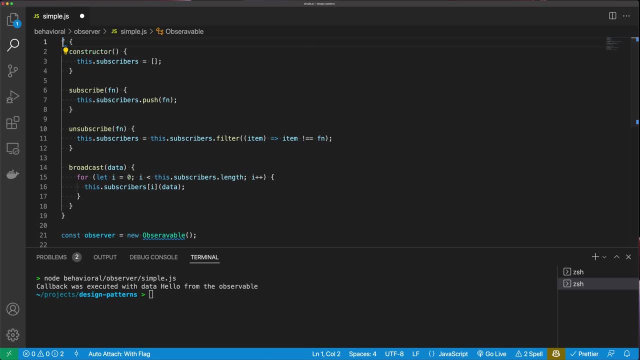 instead, because we don't like classes, so we can say function, create observable equal to. the next thing we need to do is a function is going to return an object and if you watch the previous video on factories, this syntax is going to look very familiar. this create observable is: 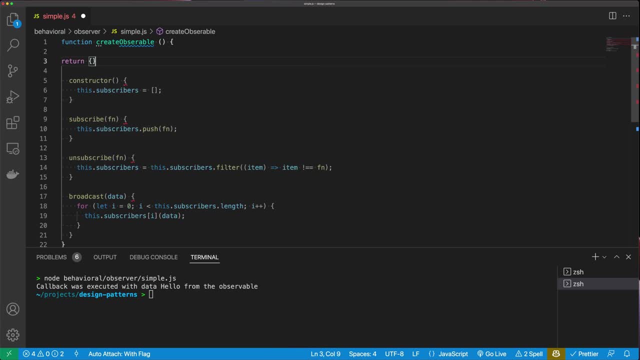 actually just a factory. i'm going to return a new object and our object is going to have subscribers so we can get rid of our constructor now, and then i can copy our methods up into the object that's returned and we just need some commas here, because it is an object so down where we create our 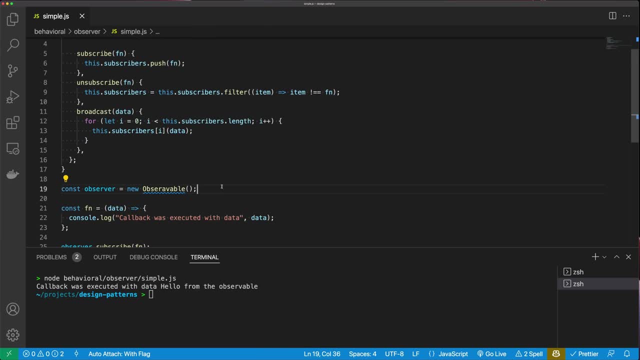 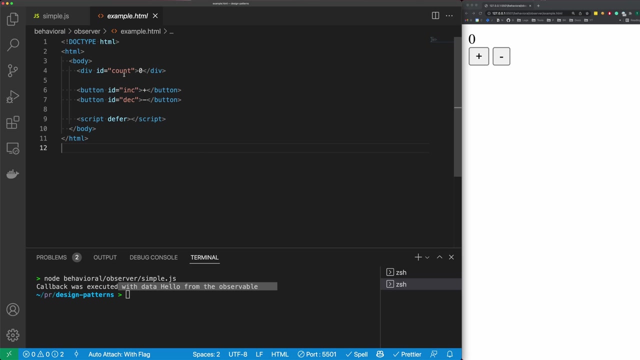 observable. we don't need to use the new keyword anymore. we can just call create observable. so our code should now output at the exact same as it did before, and it does. let's go have a look at a more practical example. example of observables. so i have this basic html page here and i have a count that starts at zero. 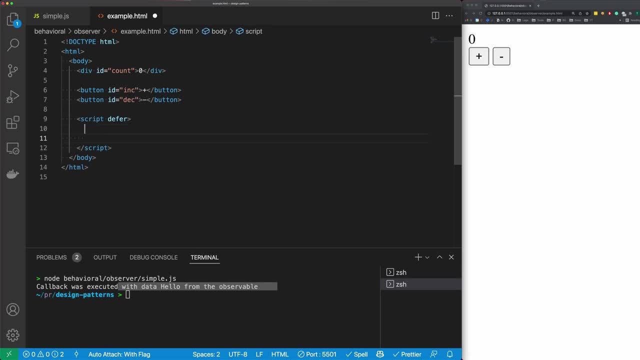 and i have an increment and decrement button and we're going to write our script inside of these script tags. here let's go over to the observable that we created before and we can just copy and paste this code that we have, and i, of course, want to create a new instance of our observable. 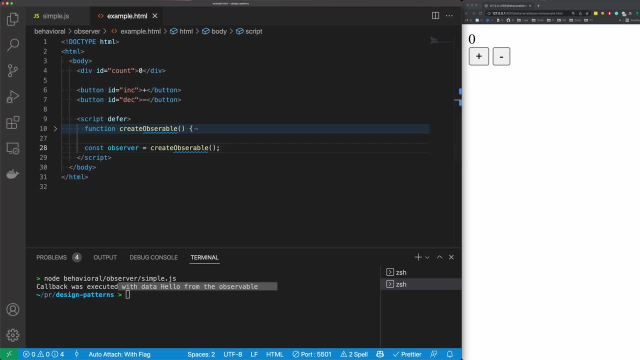 so i'm going to define a callback function. so i'm going to say function callback fn and our callback function is going to take a count, and then i just want to update our count with whatever our count is in our callback function. let me say: document dot get element. 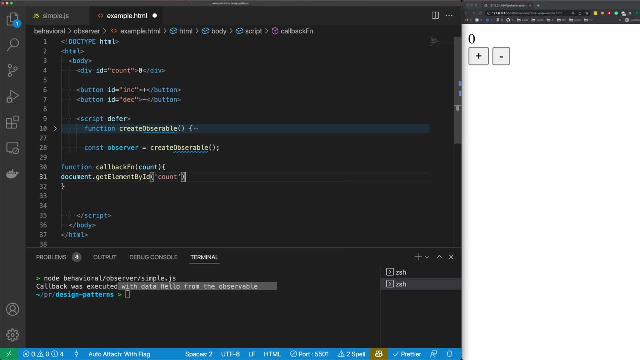 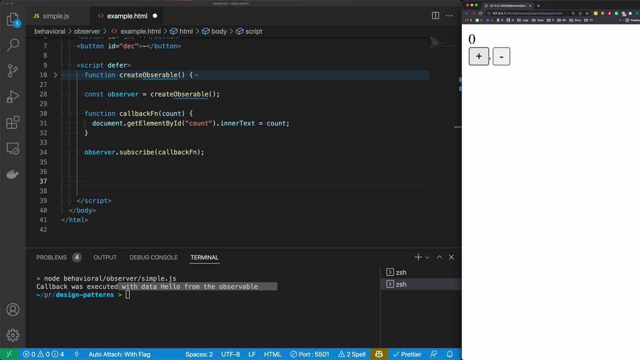 id count, dot. inner. okay, text is equal to count. the next thing i need to do is to subscribe to our observable. so i'm going to say observer, dot subscribe, and i want to subscribe with our callback function. and next we need to broadcast the messages. so whenever we click on the increment or decrement. 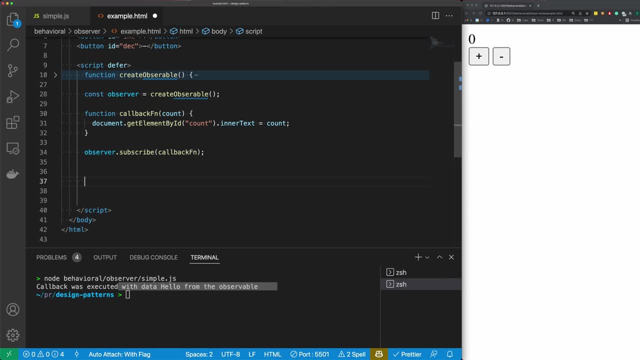 buttons. we want to broadcast a message with a new count. so i'm going to say document: dot. get element by id. inc. dot. add event listener, and this in itself is a observable. so whenever we, so whenever we call click, we're going to broadcast a message. and our observable here: 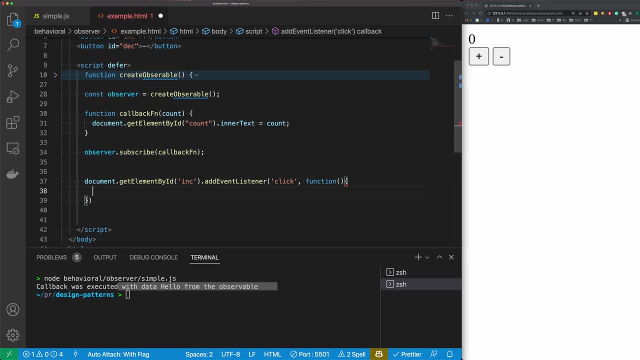 is going to listen for that message. so i'm going to provide the callback function here for the add event listener observable and i want to call observer dot broadcast and i want to broadcast a new count, so i need to get the old count first. so i'm going to say pass. 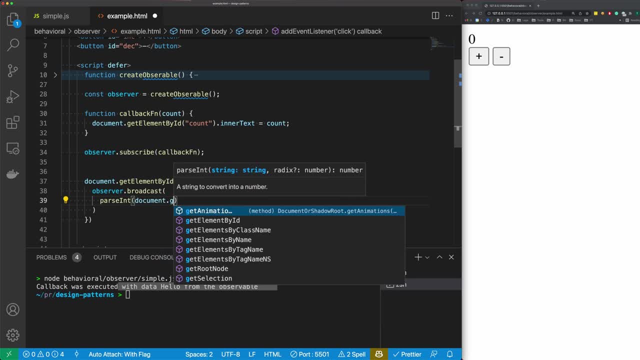 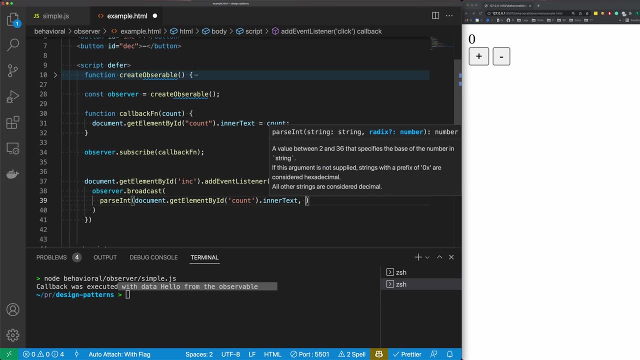 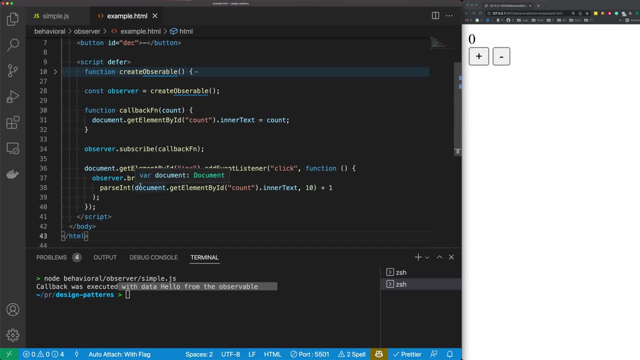 int document dot. get element by id out dot in a text and the radix parameter is going to be 10, and then i just want to be plus one. so what this is doing is we're going to get the value of count and we're going to pass it to an int, and then we're going to plus one and we're going to 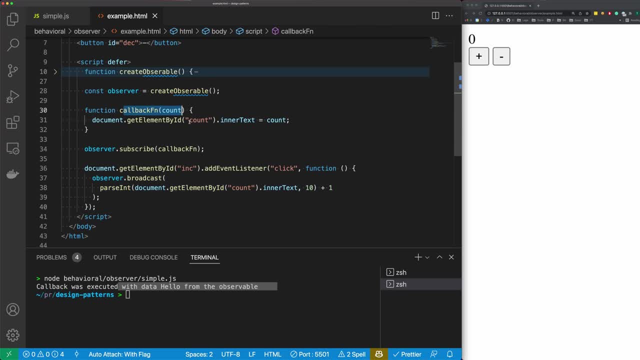 broadcast that new count out and then our callback function is going to update the count. let's try this out and you can see we're updating the count here, but we can't decrement it, so let's just copy this function here down to a new row and we just need.